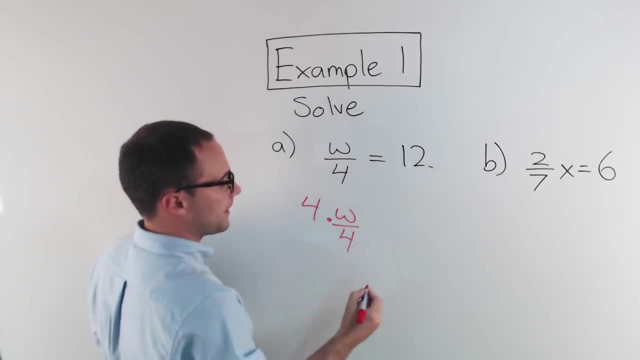 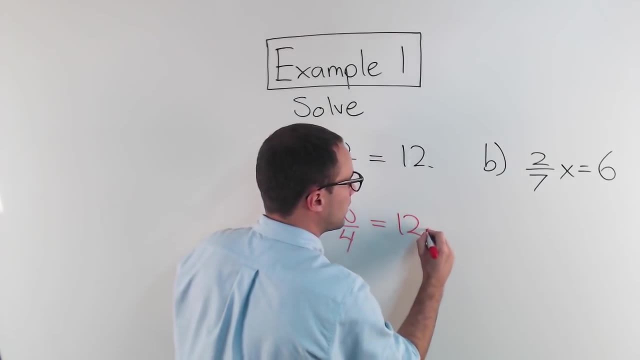 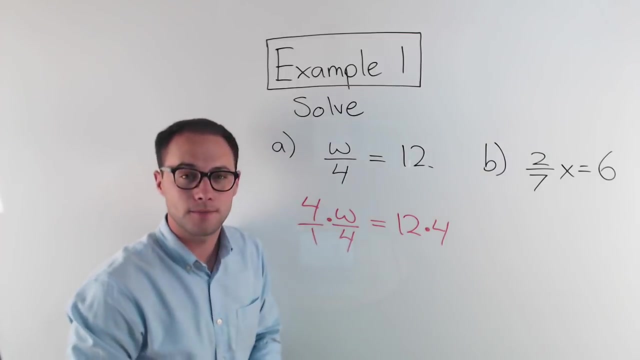 4 times w over 4 is equal to: I multiply this side by 4.. I have to do the same thing over here 12 times 4.. Okay, Well, what happens when we do that? Well, I can put that over 1.. And whenever you're multiplying with fractions, we always try to. 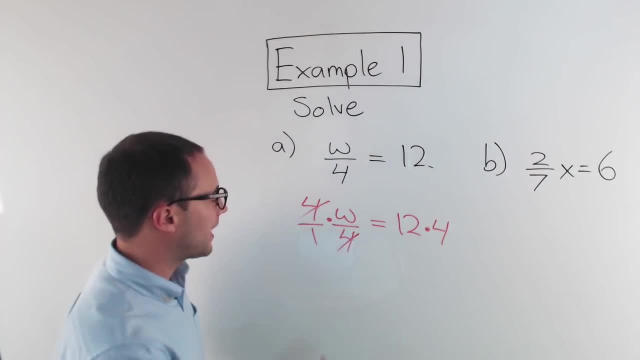 simplify, That 4 would cancel out with that 4.. And I'm left with w over 1, which is just w. That's perfect. That's what I wanted. I wanted w alone, And I have it. So w equals 12 times. 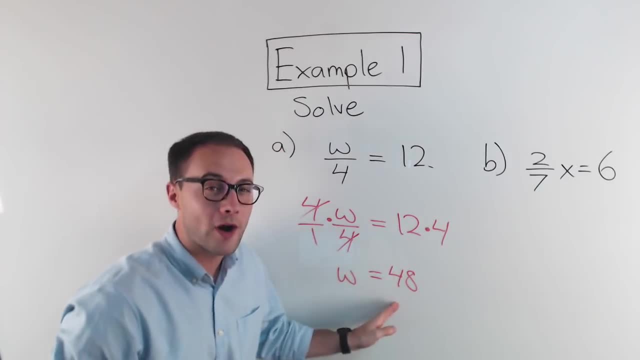 4 is 48.. Before I box that answer, I can always check. Substitute it back in at the top for w. If w is equal to 48, let's check If 48 divided by 4,, well, what's 48 divided by 4?? I can do that. 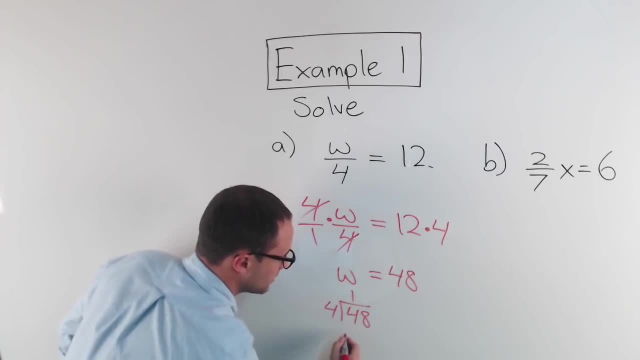 down here: 48 divided by 4.. 4 into 4 goes once That's 4.. Subtract I get 0.. Bring down the 8.. 4 into 8 is 2 times. So 48 divided by 4 is 48.. 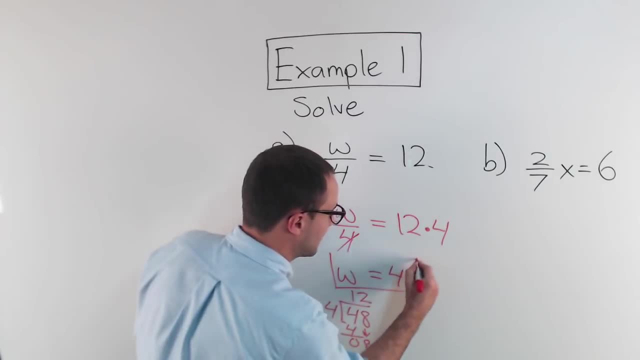 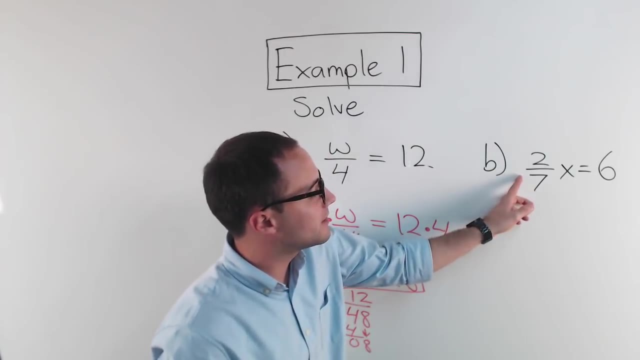 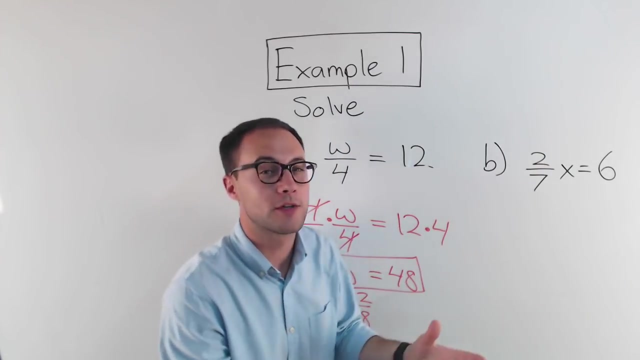 That is 12.. So that is our solution. Okay, Let's try the next one Now. we have 2 sevenths. x equals 6. This 2 sevenths is right next to my variable x, which means they're being multiplied. 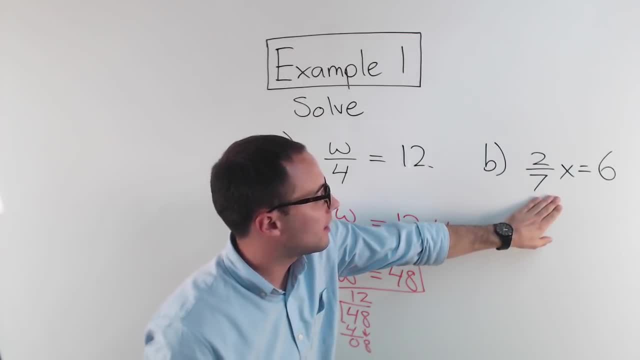 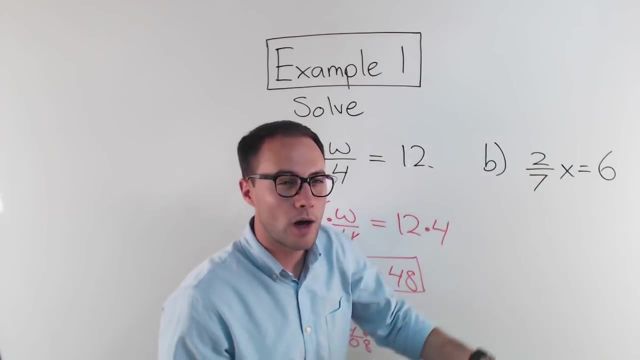 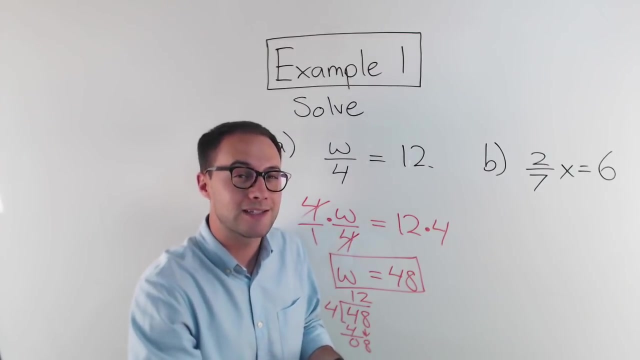 by each other. So the opposite of multiplication is division. So to get rid of this, 2 sevenths, I can divide by 2 sevenths. Well, dividing by a fraction, hopefully you remember, is the same exact thing as multiplying by its reciprocal. So what I'm 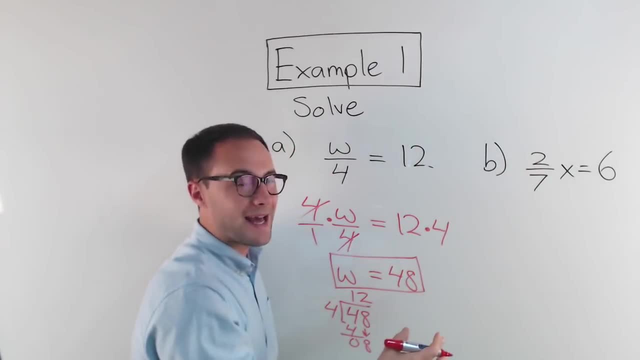 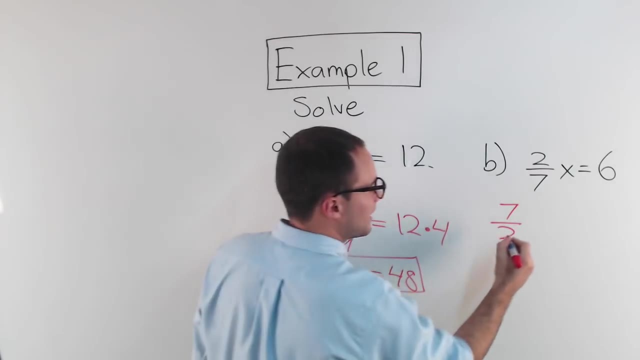 going to do is I'm going to multiply this: 2 sevenths x times the reciprocal of 2 sevenths. So I'm going to multiply it by 7 halves. 7 halves times 2 sevenths x is going to be equal to. 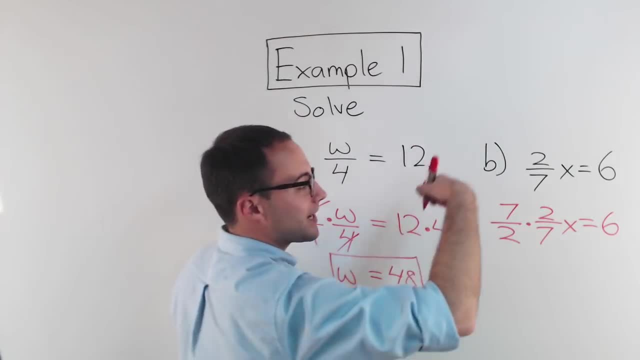 well, if I multiply this side by 2, sevenths, I got to do the same thing on the other side: 7 times 7 halves there. Well, look what happens here. Again, simplify: Well, the 2's, cancel out. 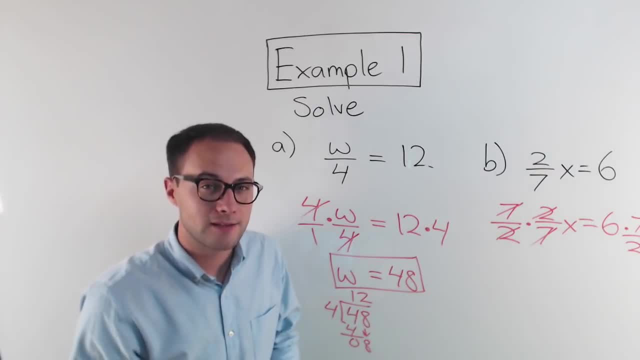 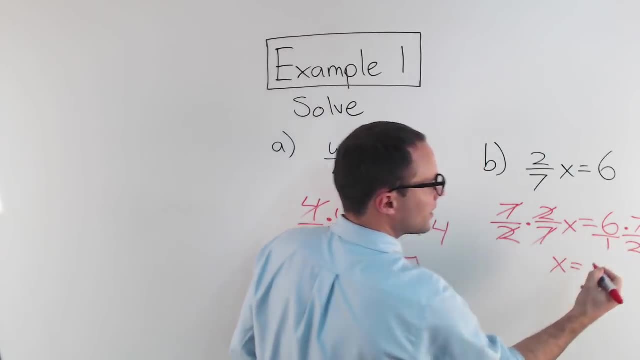 the 7's, cancel out. Basically you get 1 times x, which is just x. So I get x equals Same thing here. I'm going to try to simplify. I'll put that over 1, just so I know that it's in my numerator. 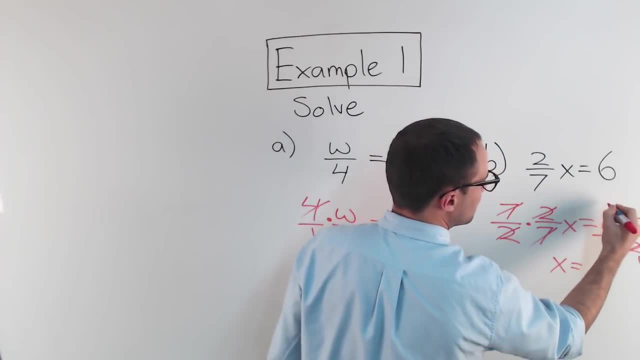 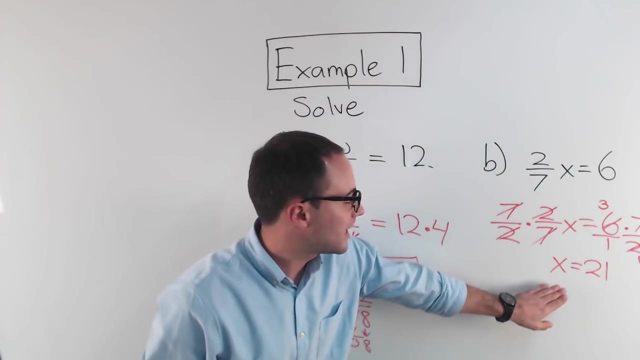 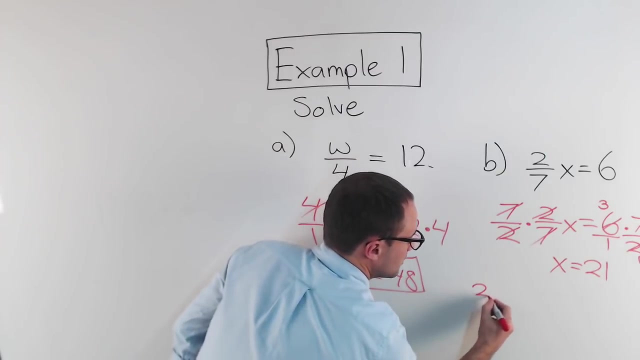 That would be 1.. The 6 simplifies to a 3.. 3 times 7 is 21.. And again, before I box that answer, I can substitute it back in 2 sevenths x 21.. Well, 2 sevenths x 21.. Put that over 1. That would simplify. That becomes what 3.. 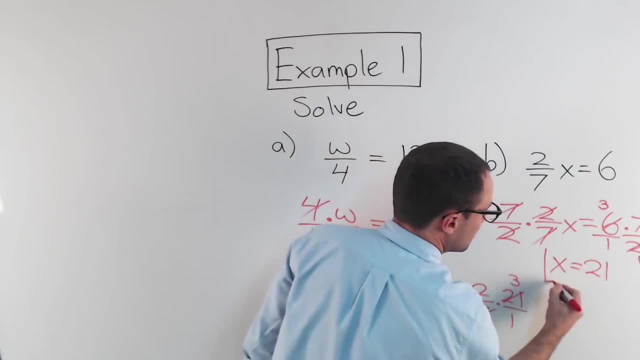 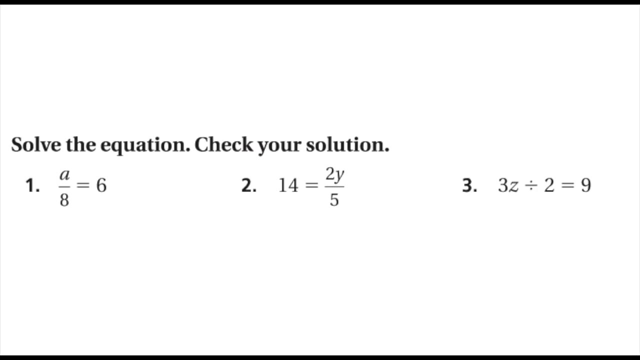 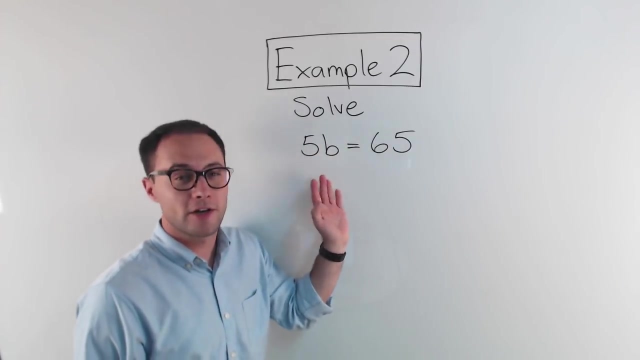 2 times 3 is 6.. So 21 is my solution. Okay, Here are some to try on your own, All right. Example 2. Solving another equation: 5b is equal to 65. Now 5b, when you see it. 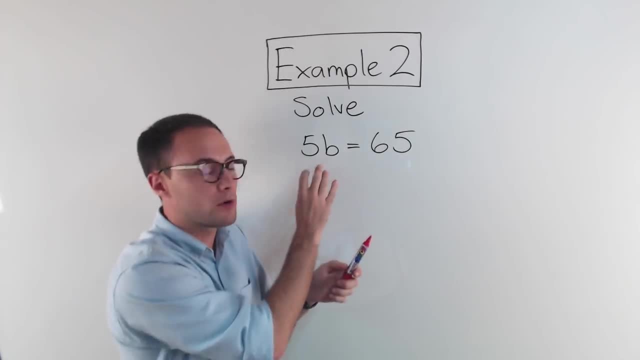 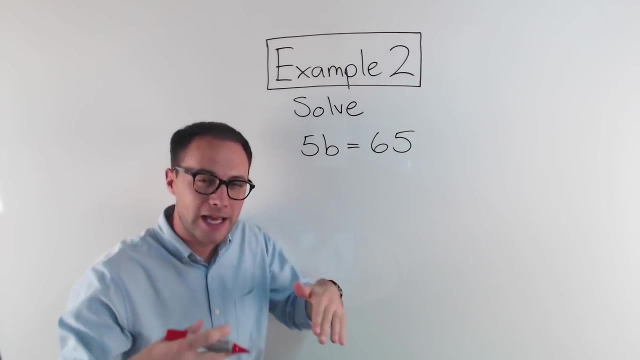 like that and you see a coefficient next to the variable. that means multiplication. This is 5 times b. So to undo that multiplication, I'm going to do the opposite: I'm going to divide. So I'm going to divide this side by 5, x is equal to 50. And here is the multiplication. 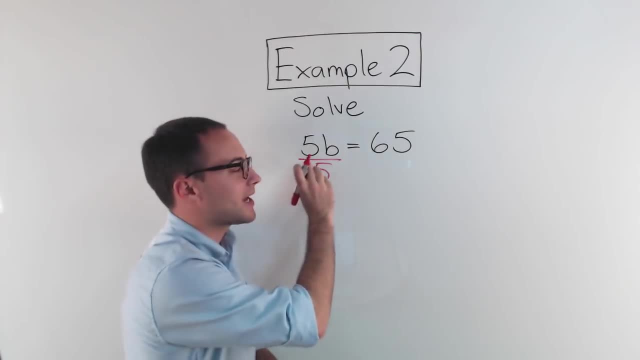 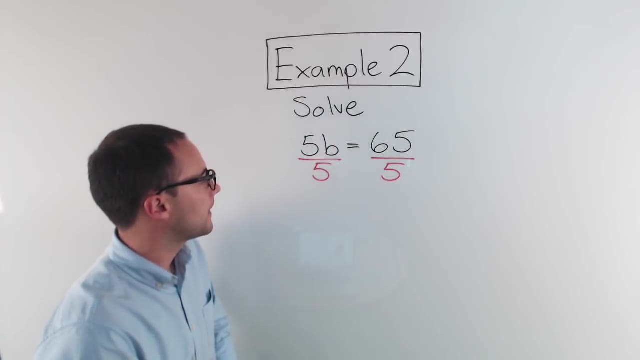 This is 5 times b. right, and anything I do to one side, I have to do to the other. so right away, I'm going to also divide that side by five, divide both sides by five. well, hopefully you notice this five and this five will cancel each other out, okay, so 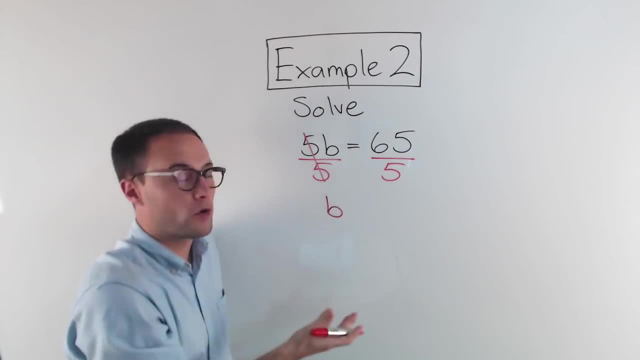 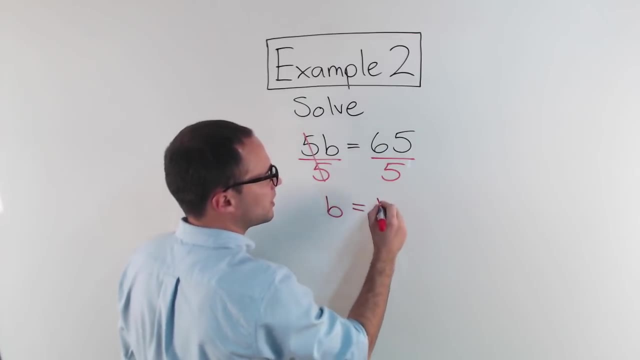 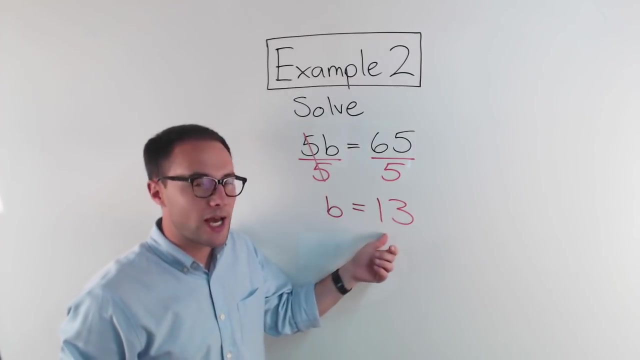 I'm left with B, which is perfect. that's my goal. get the variable alone is equal to 65 divided by 5, or 6, or 5 into 6 goes once. that's 15, so 3. so I get B is equal to 13. before I box it, I'm going to check. substitute it back in: 5 times 13 is 65. 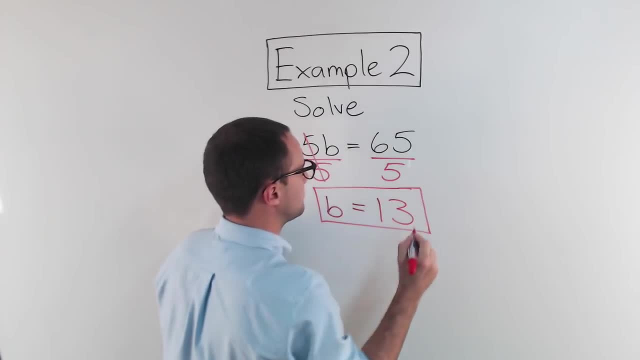 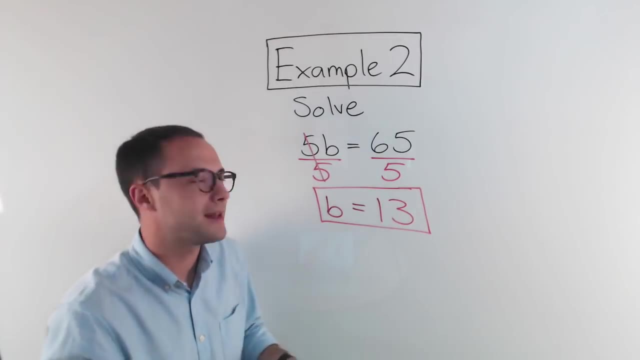 so that is my solution. okay, so here we were using division to solve this equation and write it like this: write it like a fraction. it makes a lot more difference than if you were to write it like this. it makes a lot more difference. it makes a lot more difference than if you were to write it like this. it makes a lot more. 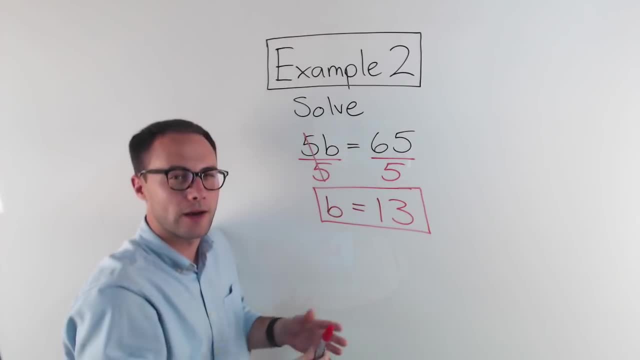 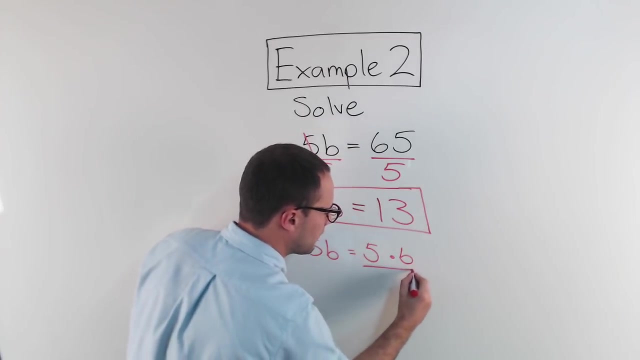 sense when you write it like a fraction, because you can see canceling out there and if you're running well, how does that leave us with B, 5 B again means 5 times B, excuse me, so if I'm dividing that by 5, well, I. 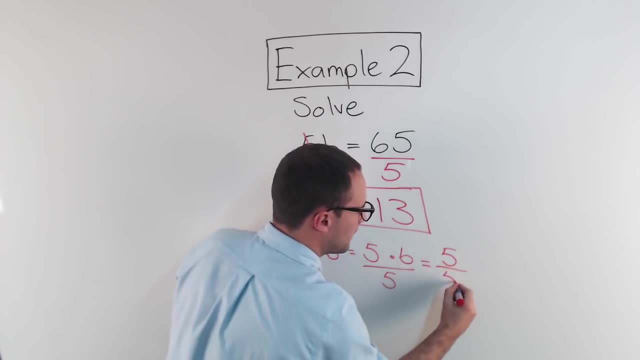 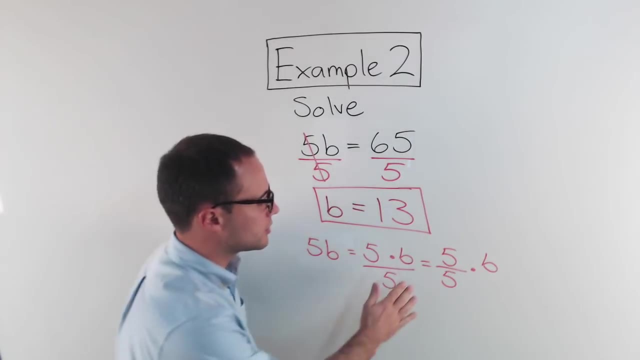 could separate that as 5 over 5 times B, right. and if you're wondering how I could separate that as 5 over 5 times B, right. and if you're wondering how I does that work, just go the other way. right, if you had 5 over 5 times B, well? 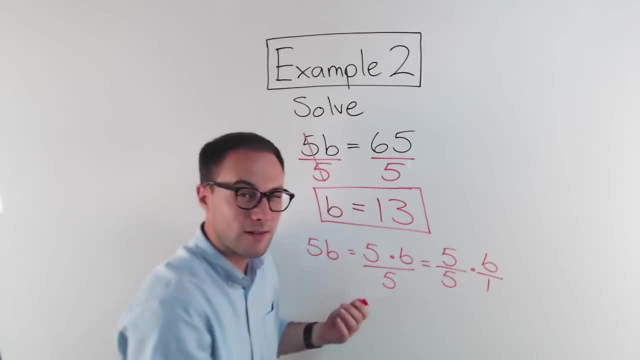 does that work? just go the other way, right, if you had 5 over 5 times B? well, does that work, just go the other way, right? if you had 5 over 5 times B? well, this is like B over 1, I can always do that. 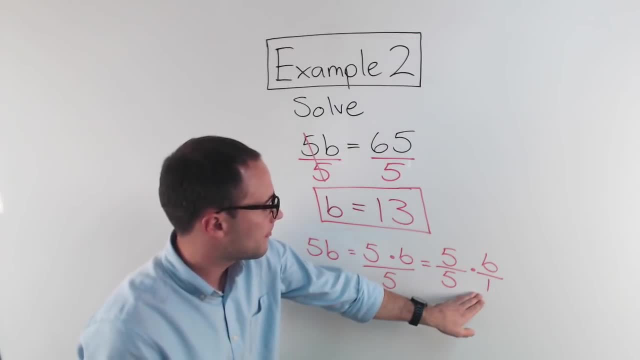 this is like B over 1. I can always do that. this is like B over 1. I can always do that with a with a variable or a whole, with a with a variable or a whole, with a with a variable or a whole number or whatever. so then I would go okay. 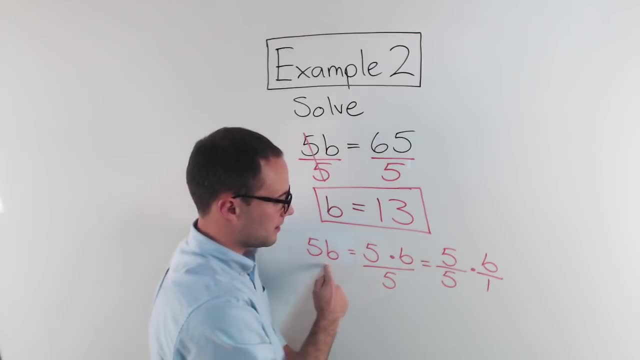 number or whatever. so then I would go: okay, number or whatever. so then I would go: okay, well, 5 times B is 5b, 5 times 1 is 5. well, 5 times B is 5b. 5 times 1 is 5. 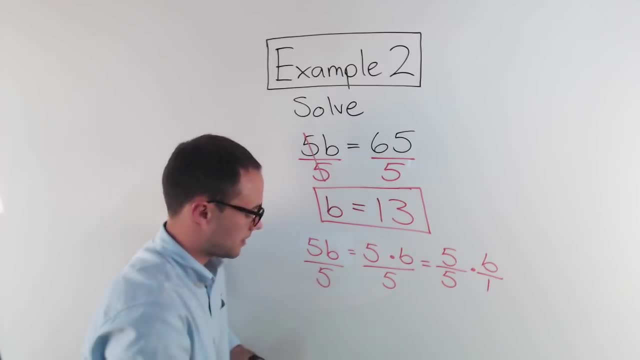 right, so I should put that down there. okay, so it's the same. and what do you get there? five over five just becomes one. that's why I kind of cancel it out with looks kind of like a big one. and then you're left with B over one, which 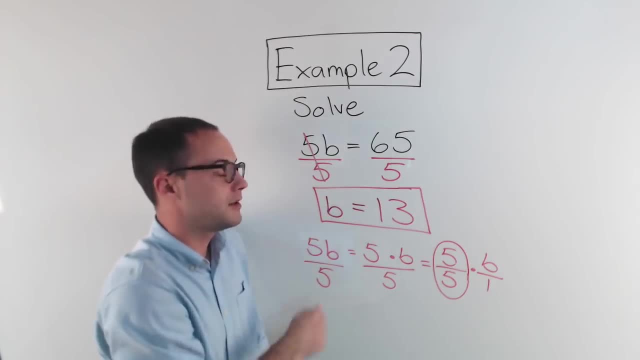 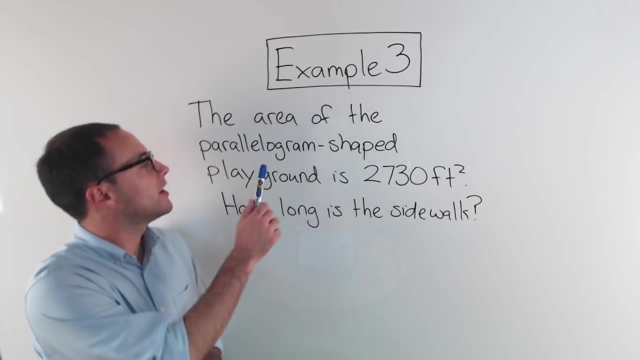 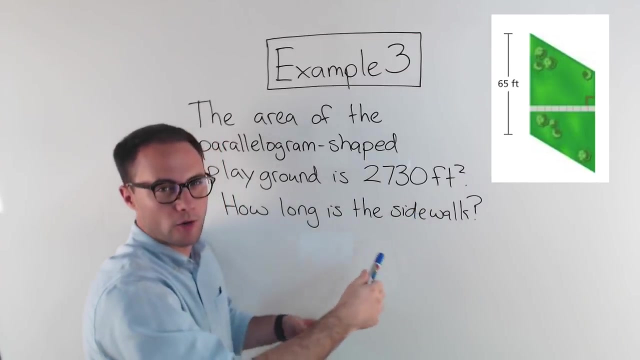 is just B. okay, so that does work you get. B alone is equal to 13. let's try one more example. all right, here's our last example. the area of the parallelogram shaped playground right over here is 2,730 feet squared, or square feet. how. 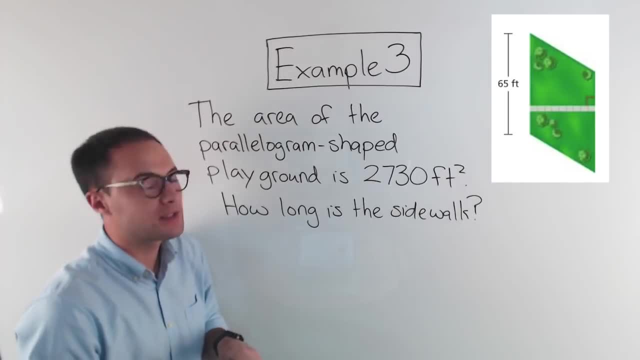 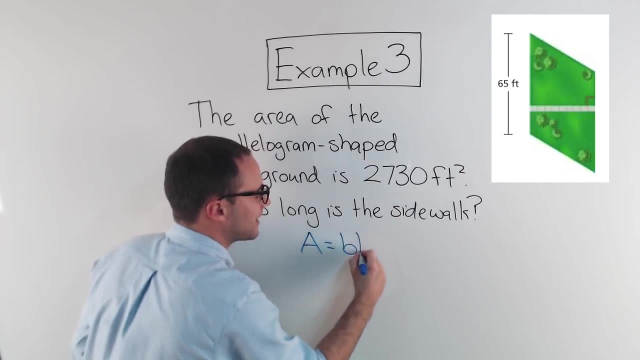 long is the sidewalk? well, if it's a parallelogram, well then we know. the area for a parallelogram is equal to base times height, and if you look at our picture, you can see that the base is 65 feet. so I can make an equation already. I. 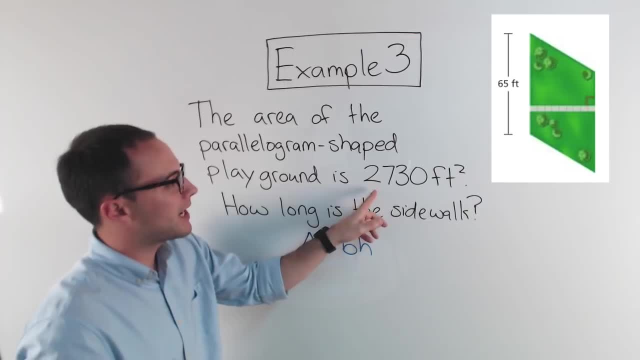 know the area of the base is 65 feet, so I can make an equation already. I know the area of the base is 65 feet, so I can make an equation already. I know the area of it area is 2730 square feet, so I'm going to substitute that in for area.